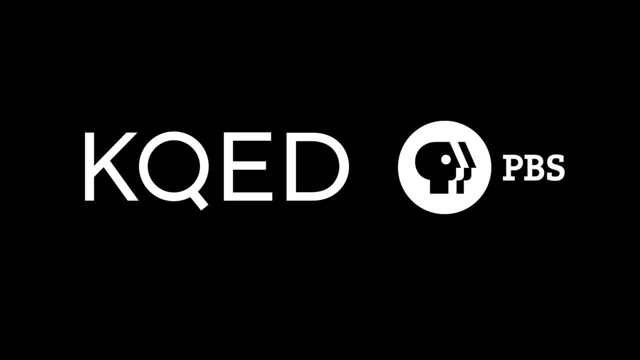 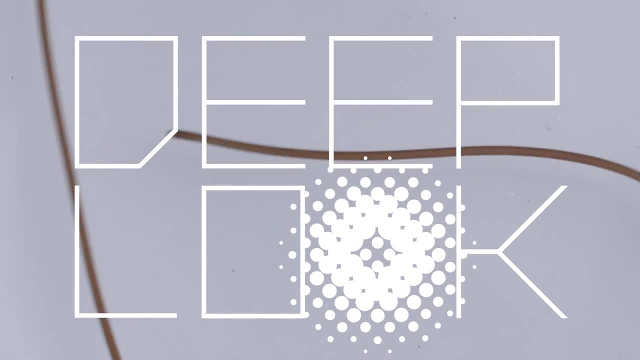 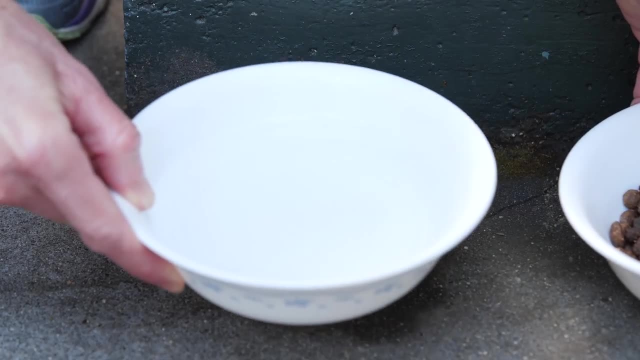 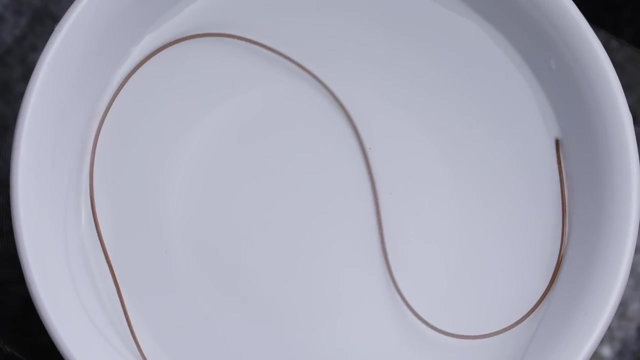 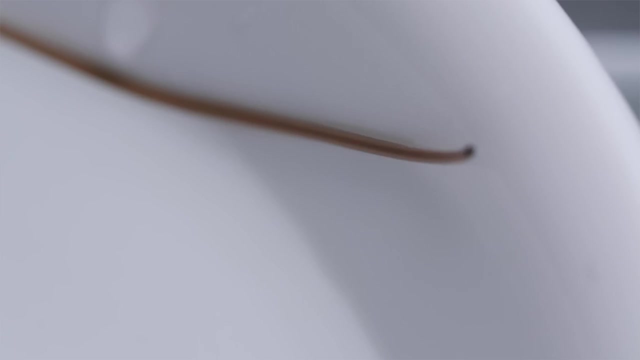 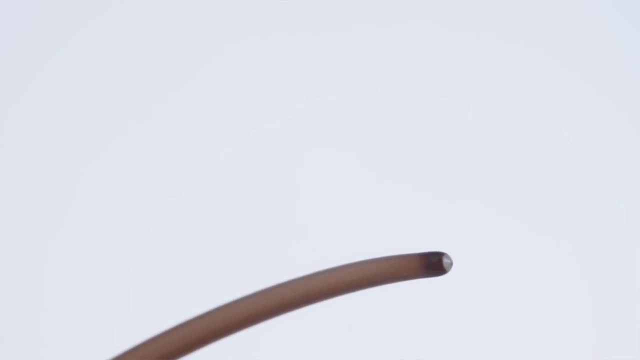 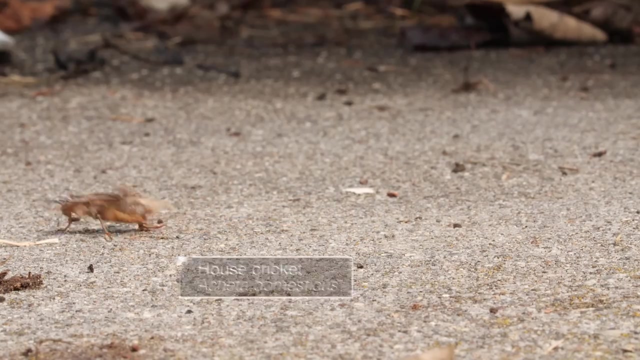 The day starts normally enough. You give your pet some food and water. But later in your pet's water dish you find this A hairworm. It didn't get here on its own. It came out of a little cricket. Don't believe me. Okay, These hairworms are gnarly parasites. They 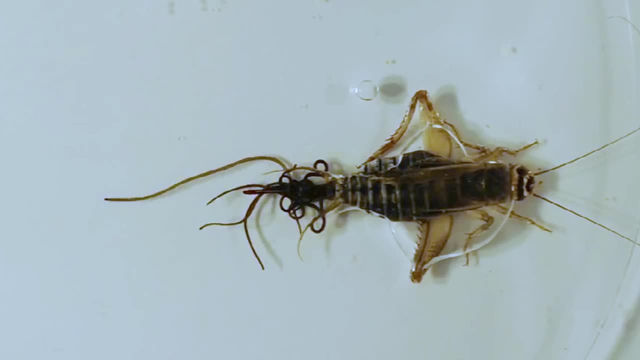 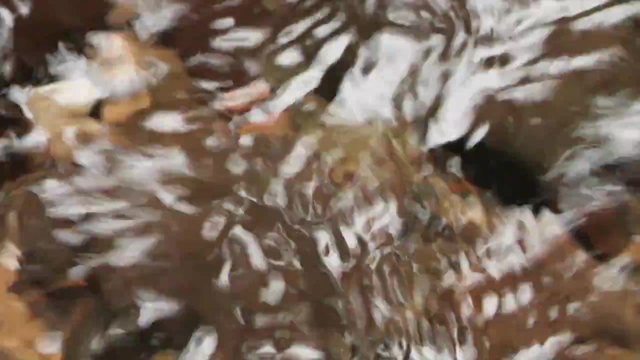 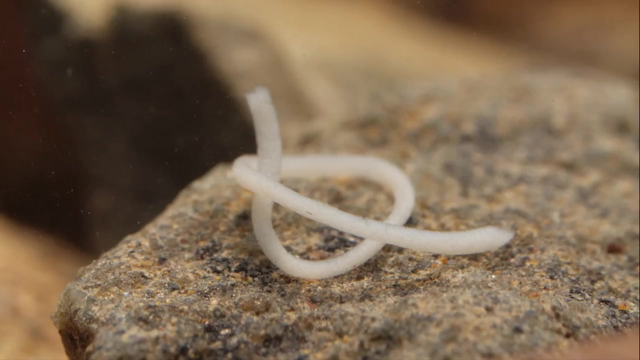 actually control a cricket's mind. to get to their home, the water, The hairworm's journey starts, innocently enough, in a river as an egg, One of many in this long string. The eggs grow into squiggly larvae, which get eaten by a mayfly larva that also lives in. 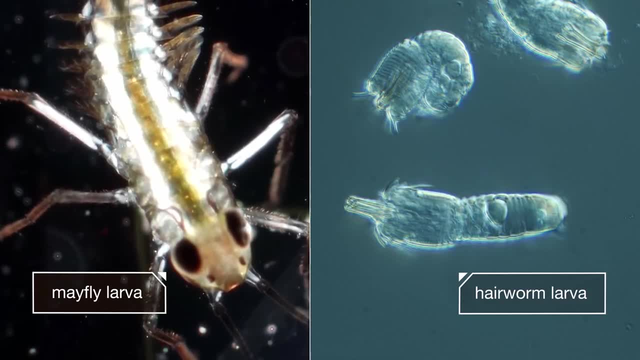 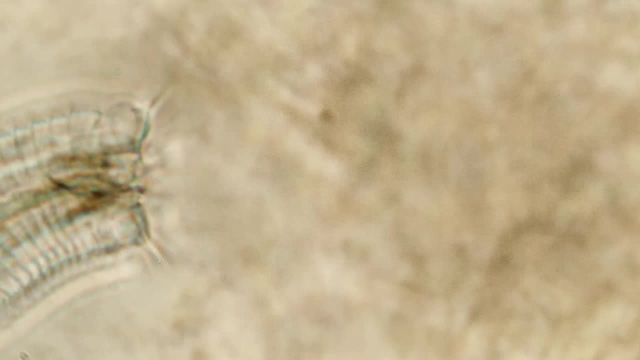 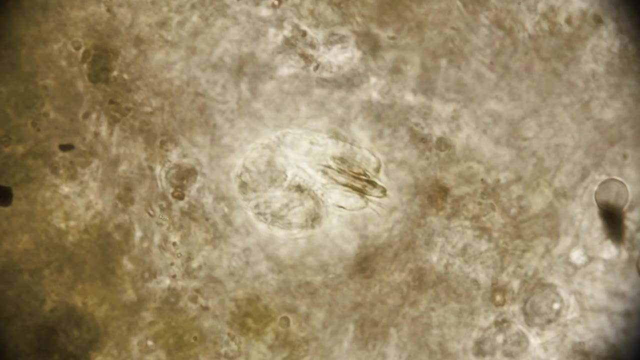 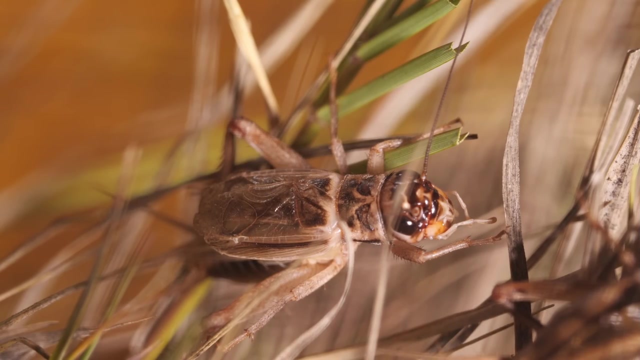 the river And inside the mayfly is exactly where the hairworm needs to be. The hairworm uses this pointy part to burrow into the mayfly's flesh. Then it curls up and waits Because really it's not after a mayfly, It's after a cricket. So it sits. 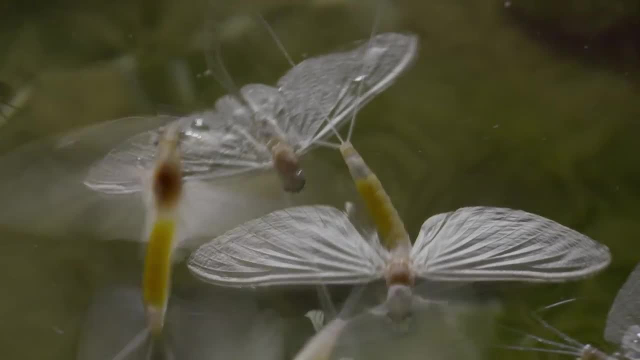 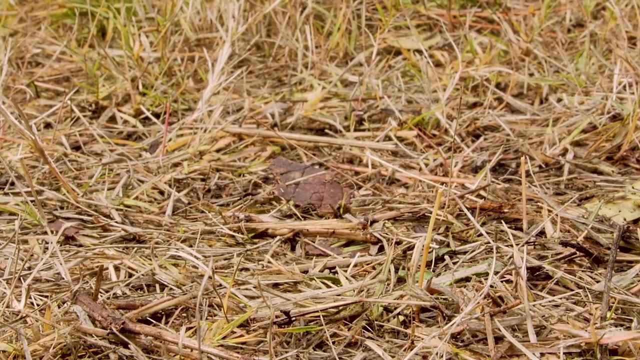 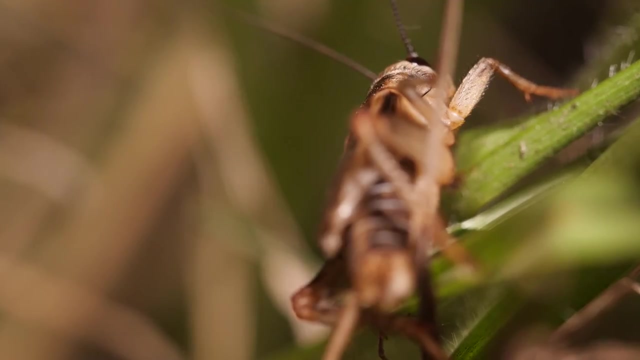 tight while the mayfly larva turns into an adult and heads to dry land, Where it just might get eaten by a cricket That has no idea what it's in for. Inside the cricket, the hairworm goes at it, Eating all the cricket's stored up fat For about. 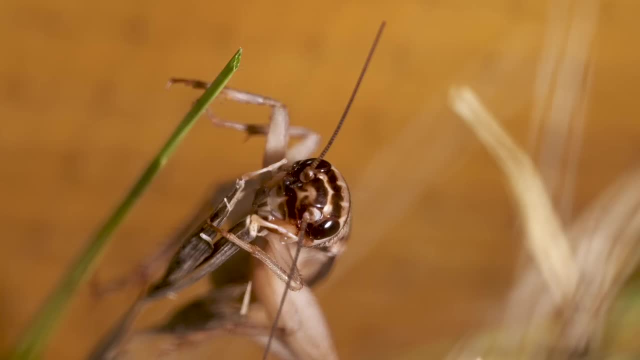 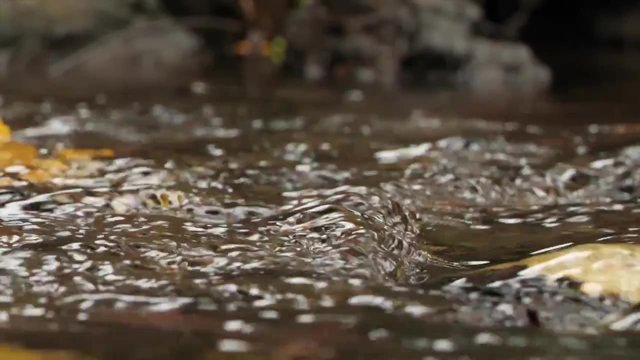 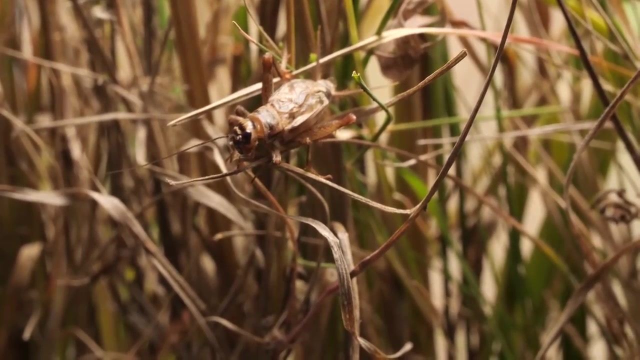 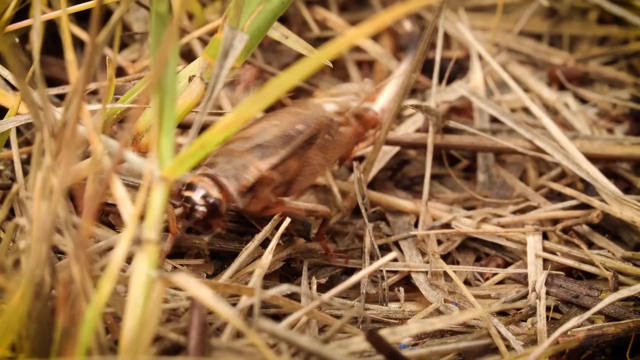 a month The cricket loses its chirp. But the hairworm doesn't kill the cricket, Because the worm needs a lift back to the water. It can easily avoid bodies of water. They're not great swimmers, So the worm takes over, Boosting chemicals in the cricket's brain which make the cricket